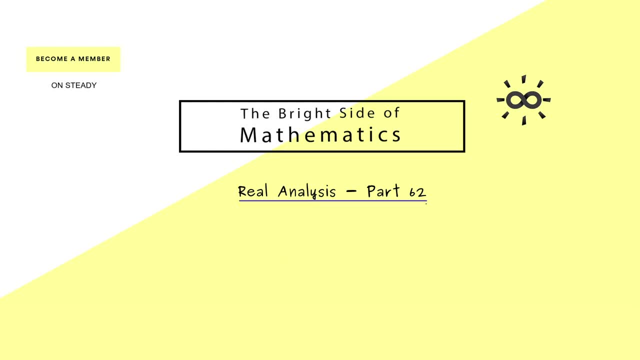 Hello and welcome back to real analysis And, of course, as always, i want to thank all the nice people who support this channel on steady, via paypal or by other means, And there, please don't forget, on steady, you can download the pdf versions and quizzes for the videos. Okay, and now in part 62, we will talk about the integral. 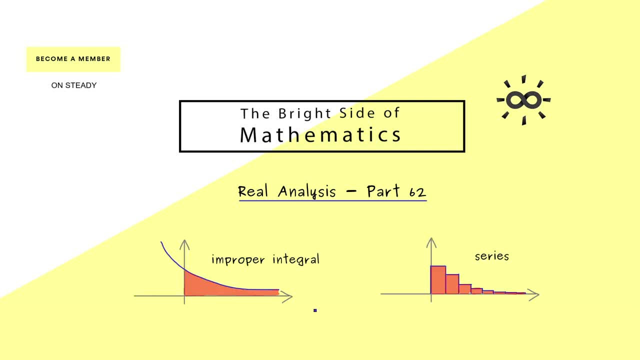 criterion for series. For this please recall that we have already introduced the notion of an improper Riemann integral that could, for example, go from 0 to infinity. In fact, in this case we immediately see the connection to a series of numbers. For example, in the last video we have: 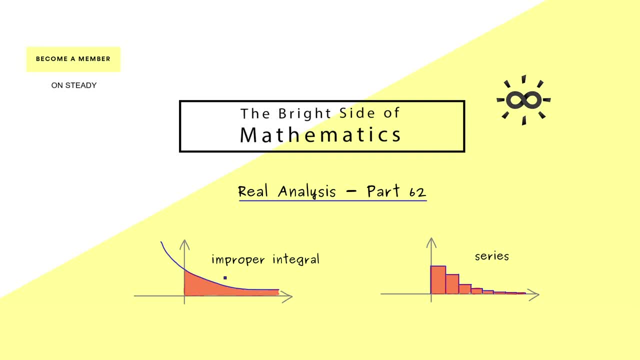 shown that the comparison test also works for improper Riemann integrals. Moreover, now we will show that we can use an integral to show that a series is convergent. Indeed, this could be helpful because for integrals we have to use a series of convergent integrals. For example, we can use an. 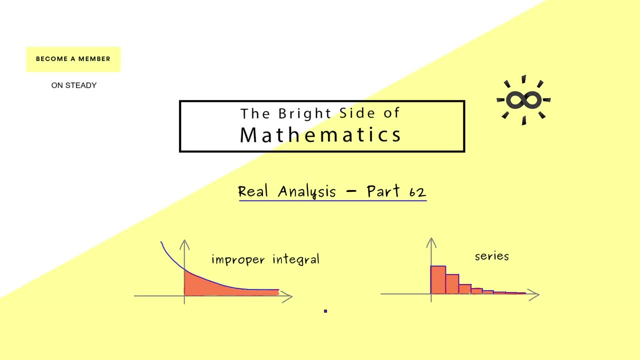 integral to show that a series is convergent. Indeed, this could be helpful because, for integrals the fundamental theorem of calculus. This means that it could be much easier to calculate a particular integral than a series. However, for having the convergence of a series, it's sufficient. 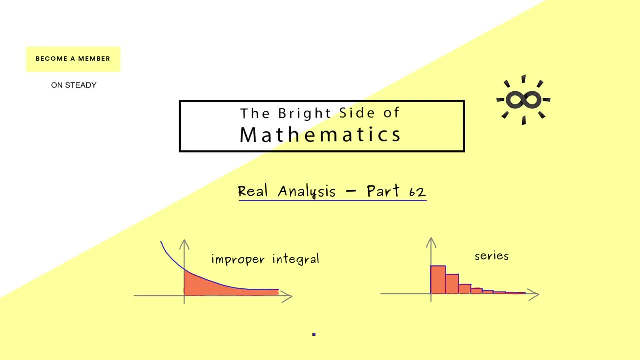 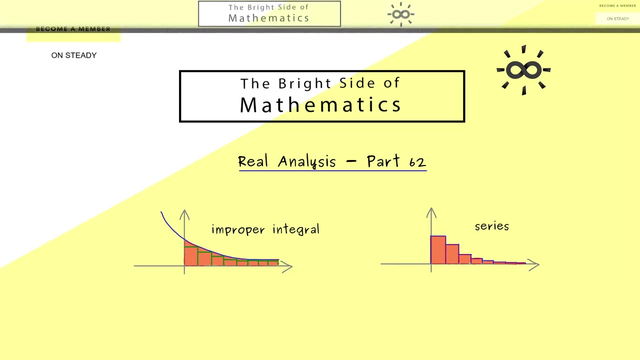 to have the convergence of a suitable integral. So maybe this is not hard to see. so assume that this area we have here on the left hand side is finite. Then when we have a series below this graph here, then the area of the rectangles should also be finite. In other words, the series then has to converge. Okay then i would say, let's. 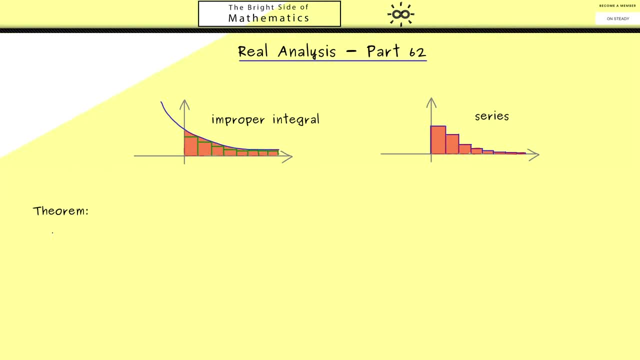 formulate this statement now. So this is a theorem often called the integral test for convergence. Now what we need is a function f with domain given by the interval 0 to infinity, which is also non-negative. So we could write that the codomain is also the interval from 0 to infinity. 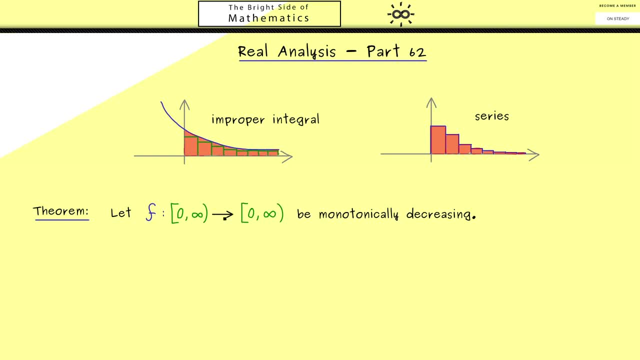 However, we could also write that the codomain is also the interval from 0 to infinity. However, we also need, as you can see in the picture, is that the function is monotonically decreasing. Okay, that is all we need, and then we can conclude that the series from k is equal to 0 to infinity. 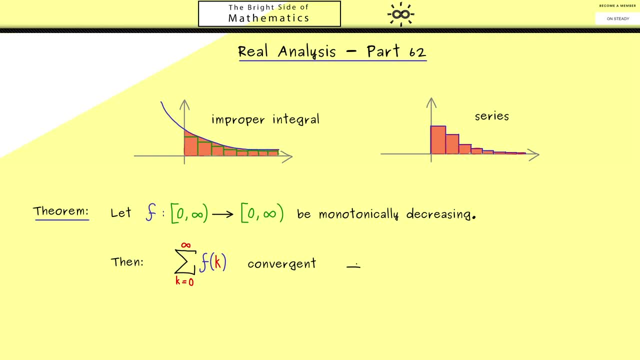 of f, of k is convergent if, and only if, the improper Riemann integral is convergent. Hence, if we know that this integral gives us a finite number, then this series also gives us a finite number. And if we know that this integral gives us a finite number, then this series also. 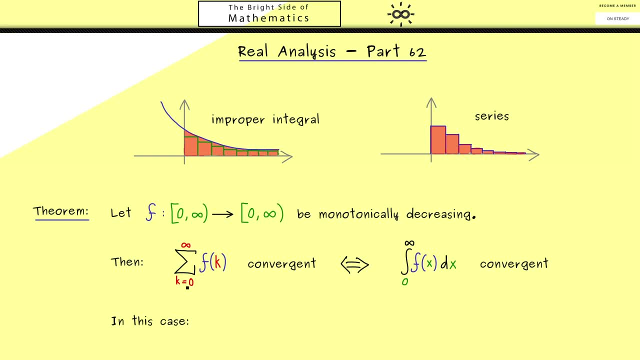 gives us a finite number and vice versa. And, moreover, in this case, we can estimate the values. First, we see that the series is always larger than the integral. Therefore, the difference is greater or equal than 0. And maybe this is something we can explain in a picture. 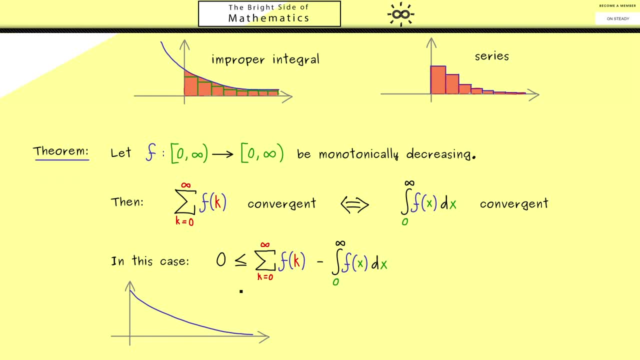 Now, if this is the graph of the function f, the series is evaluated at the integers, at the x-axis, For example, f of 0 would be this value, f of 1 has this value, and so on. Now, adding up all these values is the same as adding up the areas of rectangles, because the 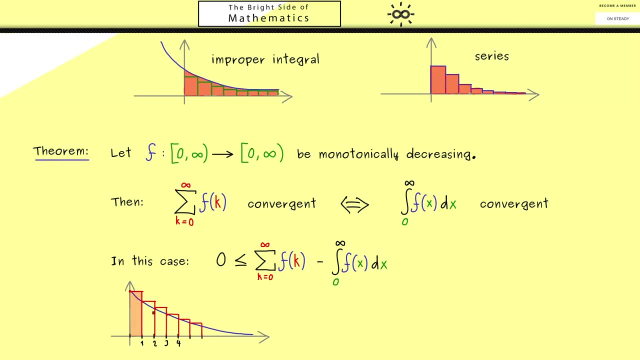 width is 1.. Then the important thing you should see is the area is larger than the integral. So you see, this immediately explains the implication from the left to the right And also this inequality here. Now, in order to explain the other implication, we have to look at the picture again. 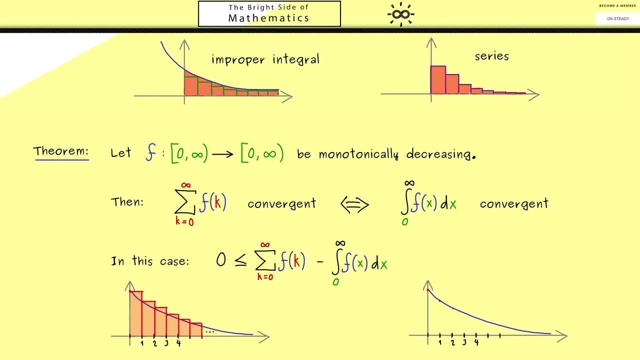 Of course we still have the same values here, but now we have another idea. Instead of drawing the rectangles to the right, we could draw them to the left. Then the first one, for f of 0 would lie outside the area of the integral, but this is no problem. 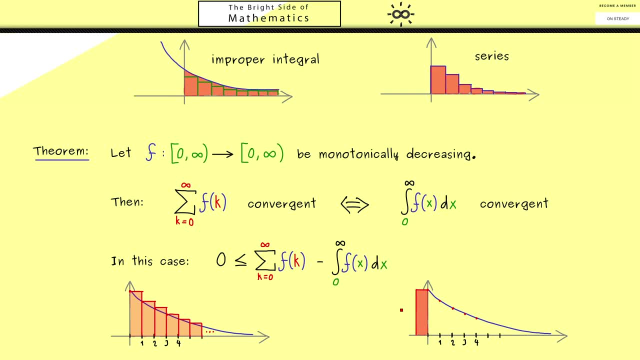 at all. It's a finite number, which means we could ignore it, and this means that we start with. the series at k is equal to 1.. Hence then we see that all the other rectangles lie inside the integral area. In other words, the sum of all the rectangles is less than the integral of f. 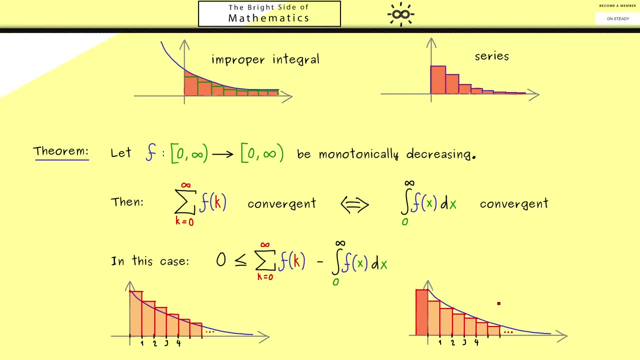 And there we see, there we have the other implication. Hence, if this integral is convergent, then the series starting with 1 is also convergent. However, then starting with 0 is, of course, also convergent. Moreover, from this we can conclude that the 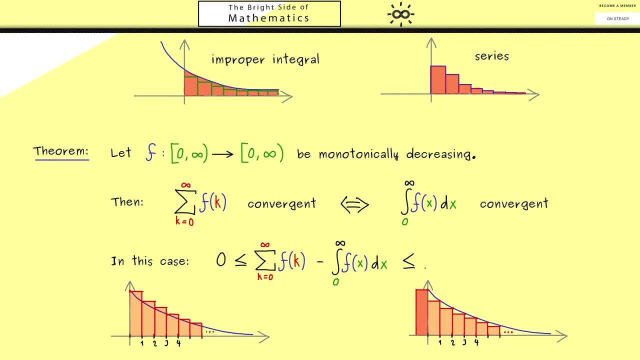 difference here cannot be larger than the first entry, In other words the value of f at 0.. Ok, and with this the formulation of the theorem is finished And in some sense, as you can see, we already explained the proof of it. However, i would say let's do it again in the formal correct way. Still, it's a good thing. 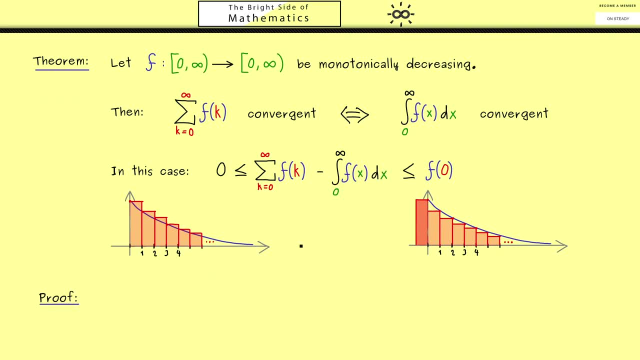 that we already have the ideas we need. For example, we know that f is monotonically decreasing. From this we can conclude that for all k greater than 1, we have that f of k is less or equal than f of k minus 1.. Moreover, all other points x between k minus 1 and k also fulfill this. 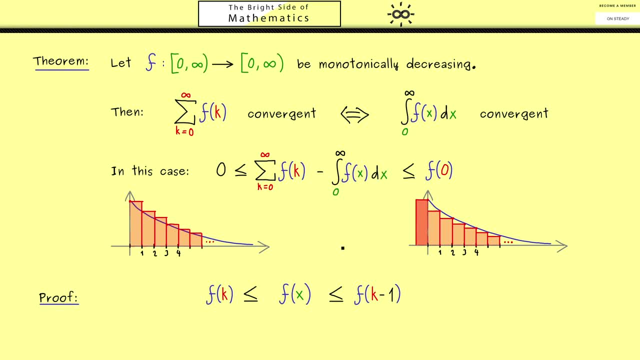 inequality. So we immediately get this from the monotonicity, And now we know that the integral conserves such a monotonicity. Therefore, we can put an integral sign on all sides of the inequalities. However, now, of course, we only integrate from k minus 1 to k. There, please, 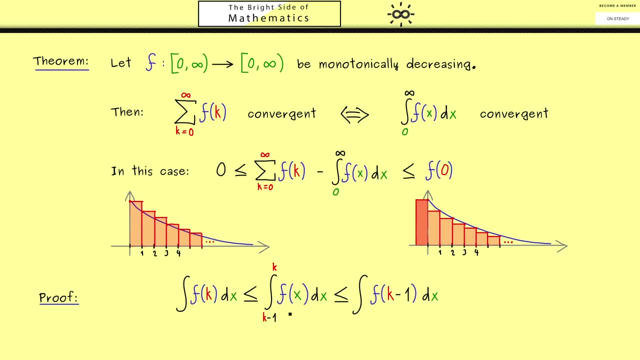 recall, x needed to be in point from this interval. So in summary, the monotonicity of the function f gives us immediately these nice inequalities for the integrals Also. you should see, here on the left hand side We have picked a rectangle here and here on the right hand side we have picked a rectangle. 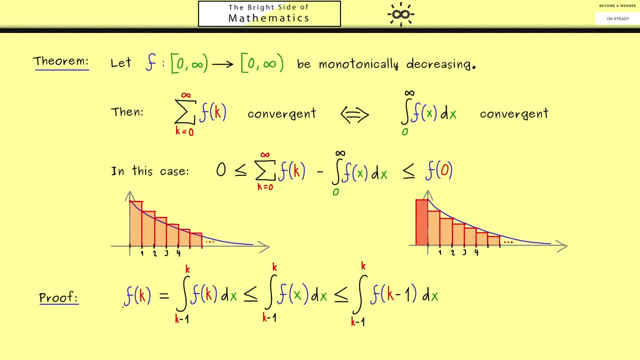 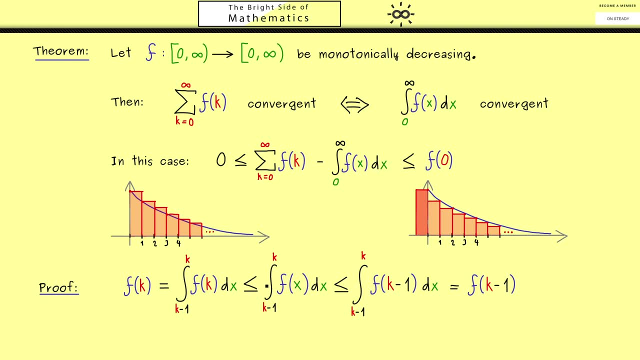 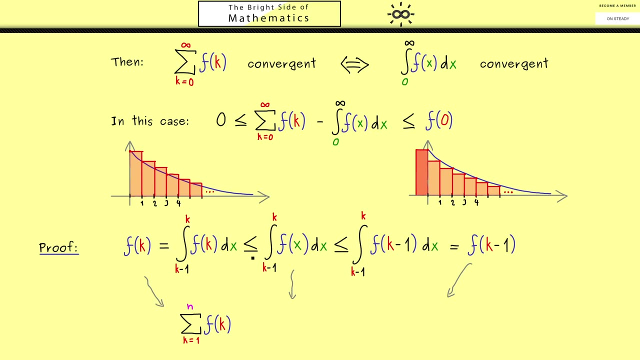 there. In other words, this is simply the value f of k, and on the other side, we have the value f of k minus 1.. Therefore, in the next step, we can sum up all the rectangles. Of course, when we start with 1 and go to n, we don't change the inequalities Indeed. now we see. 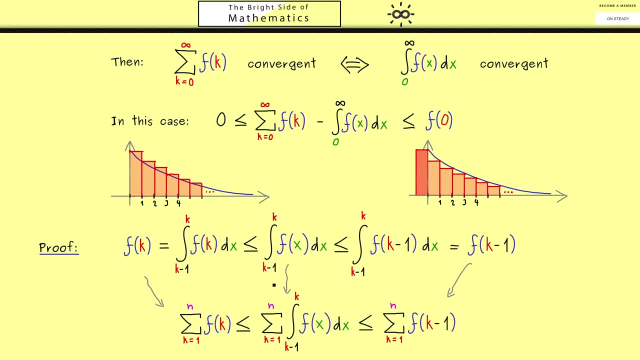 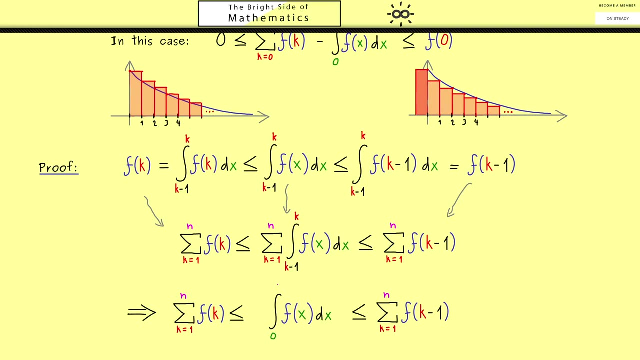 the inequalities of the pictures. again, In the middle we have the area given by the integral, and on the left and the right hand side we have the rectangle summed up, Therefore, i would say let's formulate this in a nicer way. First, the middle part. here we can write as the integral from 0 to n. 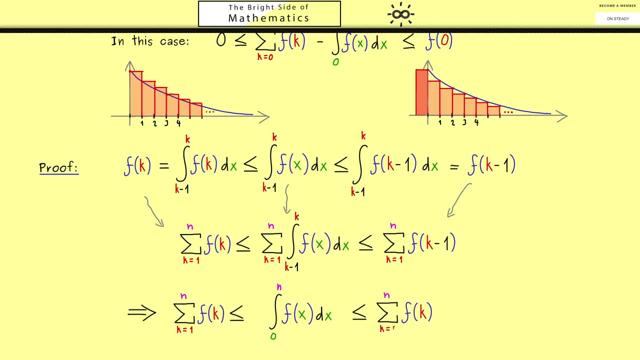 And for the right hand side, we can write f of k, and then we start at 0 and go to n minus 1.. And then you should see, we have everything we want, Namely when n goes to infinity- And this here gives us a finite value- then this is also a finite value. 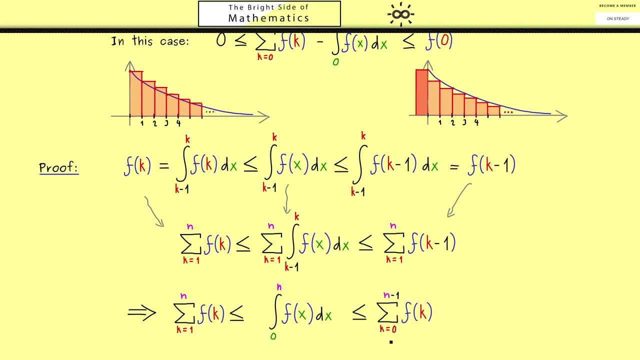 On the other hand, if we send n to infinity here on the right hand side, and this series gives us a finite number, then this integral in the limit also exists. Therefore we could say, while considering these limits, n to infinity- the first part is shown, Then the second part was the inequality, and this comes also out. 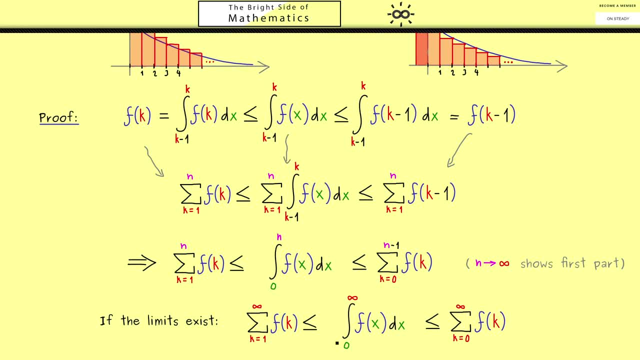 More precisely, If the limit exists, we have these two inequalities where on the left hand side we have the series starting at 1 and on the right hand side the series starting at 0. Hence, by subtracting the series here, we get the two estimates from the theorem. 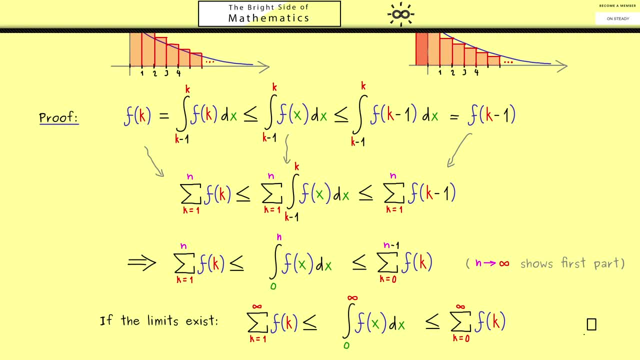 So, in summary, everything is formally proven now. So you see, the proof was not so hard, but the statement is something you really should remember. Therefore, i think it's a good idea to look at an important example, In fact this one you really should remember. 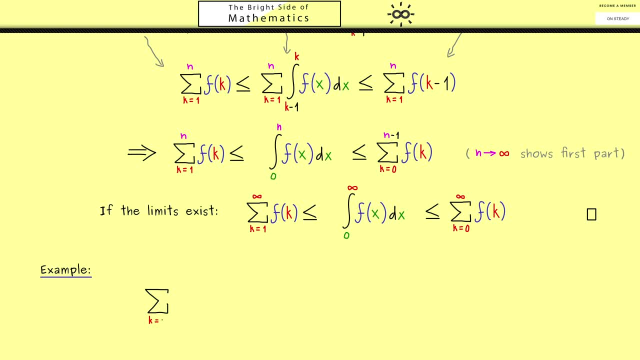 Here we look at a series that starts with k is equal to 1.. This means that the corresponding integral should also start at 1.. Of course, it's no problem at all to adapt the theorem to this case. And now the series we consider is 1 over k to the power alpha. 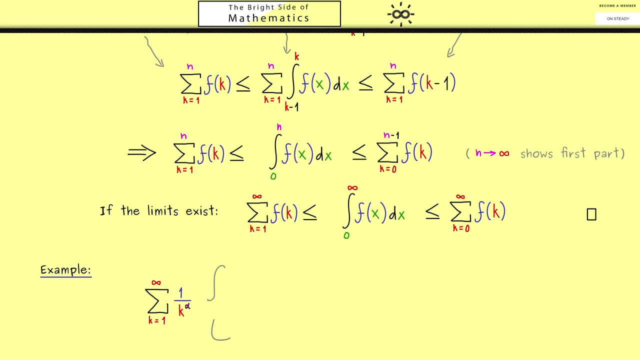 And now, depending on the value of alpha, we get two cases. Namely, we get a convergent series When alpha is large enough, which means alpha should be greater than 1.. And, on the other hand, if alpha is less or equal than 1, the series is not convergent. 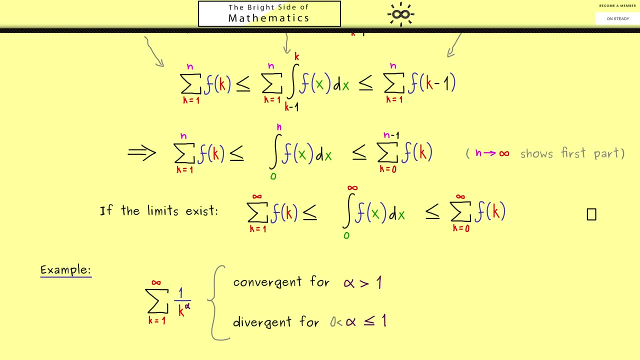 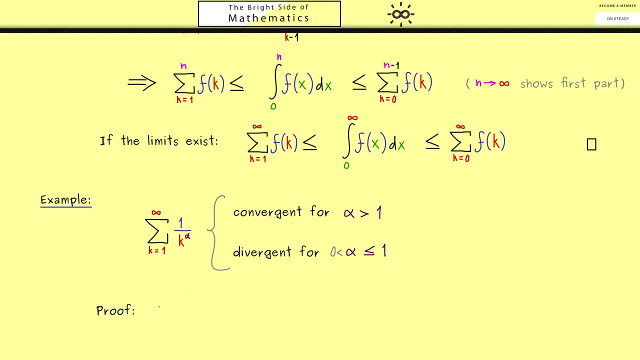 Of course, if you want, you can assume that alpha is positive, Simply because if alpha is negative, it's very clear that the series can't be convergent. Ok now, this statement here we can prove by using an improper Riemann integral. And, of course, 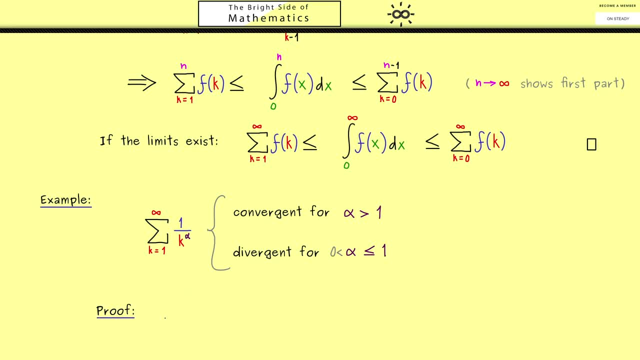 The function in the integral should be 1 over x to the power alpha. And there you see the good thing for this integral. here is where we integrate from 1 to b that we know an antiderivative for the function. More precisely, we have to distinguish two cases. 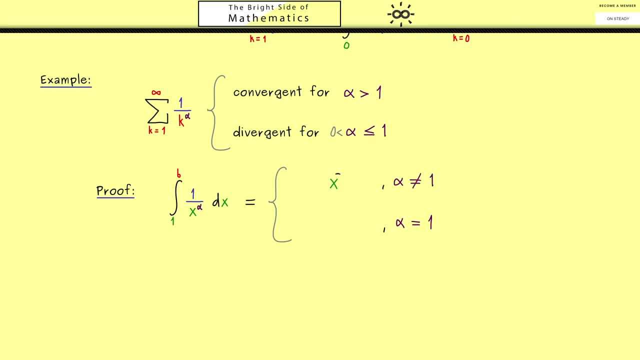 Now, if alpha is not 1, the antiderivative can be written as the function x to the power minus alpha plus 1.. Because now the derivative of this function gives us x to the power minus alpha, which is 1 over x to the power alpha. 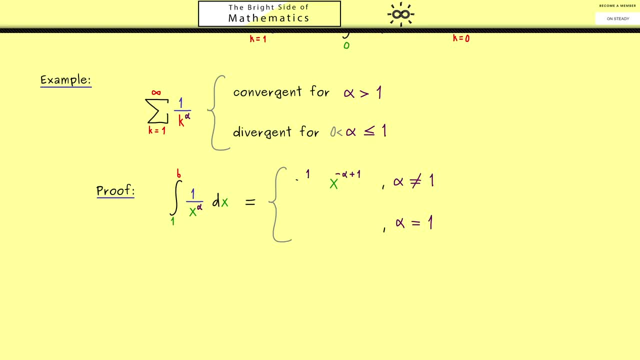 Therefore, you see, we only have to fix the constant, the factor that comes in front. Obviously, this is also minus alpha plus 1, but I write it as 1 minus alpha, And there you see, this whole thing does not work. for the case, alpha is equal to 1.. 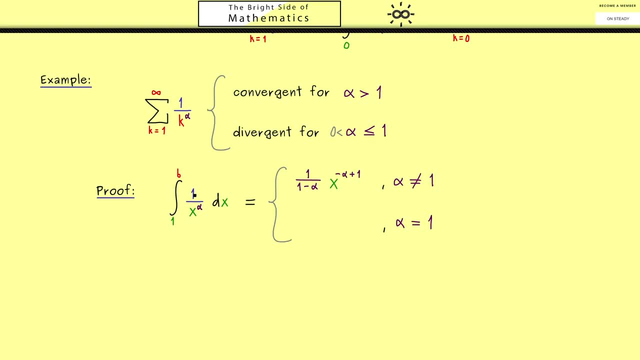 However, there we only need to know the antiderivative of 1 over x, Which is, as you might know, the natural logarithm. Ok, and now. both antiderivatives are evaluated at b and 1.. Ok, then lets do it and put in b and 1.. 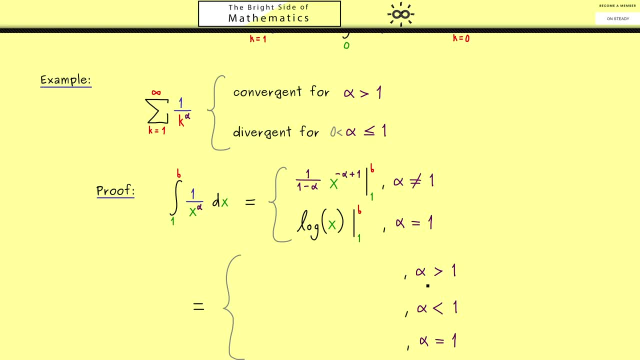 But then I want to distinguish the first case with alpha is greater than 1 and alpha is less than 1.. Ok, of course its not so complicated. we put in b and then we subtract, putting in 1.. However, now I want to make it clear that this power is negative. 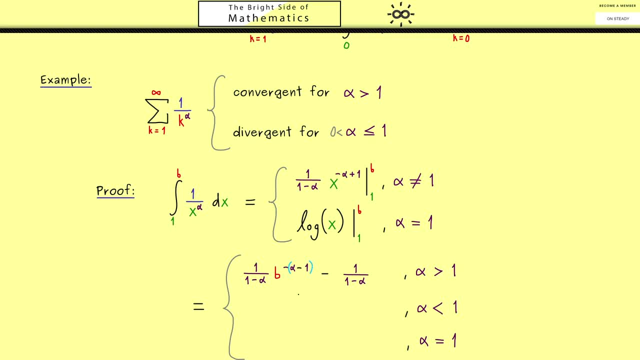 So when I put parenthesis here, we have a minus sign here. Ok, now more over. for the second case. we have the same result, of course, but now the power is positive. So lets make this clear by putting 1 in the front. So we subtract something that is always less than 1. therefore, the power is always positive. 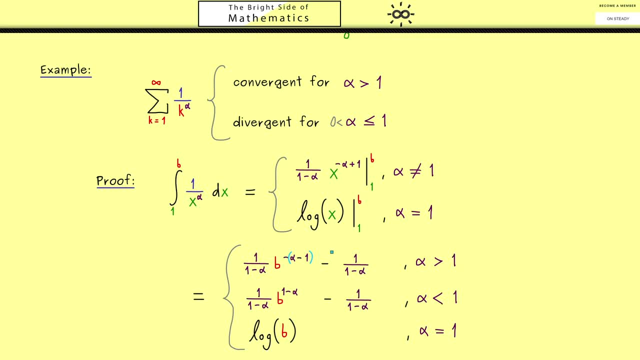 Ok, then in the last case, you see we just have log of b, And now the question we should answer is: what happens when we send b to infinity? Now, in the first case, because we have a negative power, this one vanishes and only this term remains.